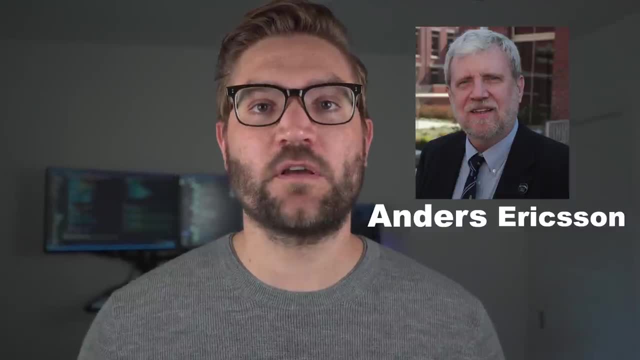 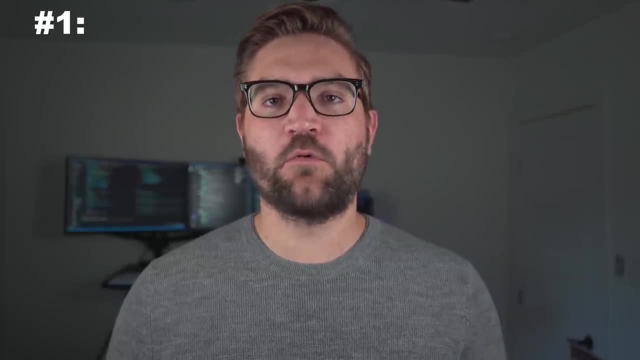 whose research really focused around expertise and human performance, coined this term: deliberate practice. Now I've simplified the key parts of deliberate practice that are going to be important for you, and they are as follows. Number one: deliberate practice requires that you have clear and well-defined goals. So that means when you sit down to study or practice. 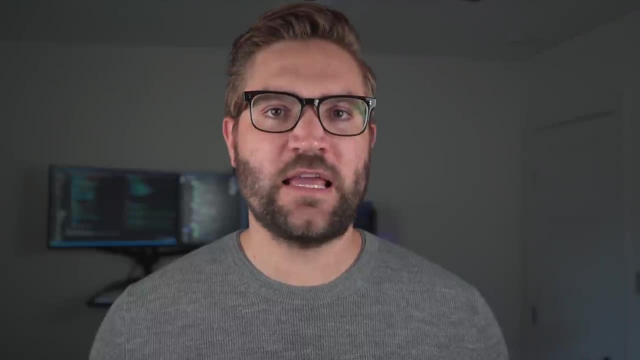 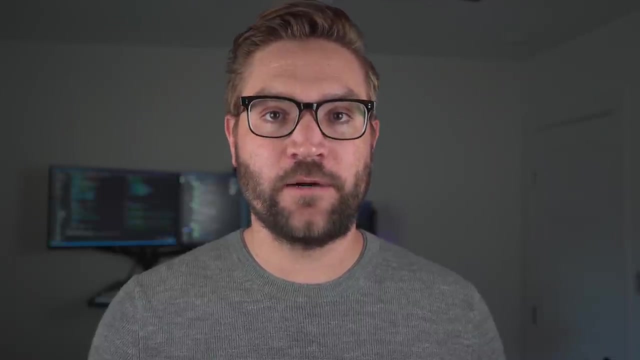 what skill exactly are you trying to improve? It could be as simple as saying: I'm working on my problem solving skills. That's why I'm building this portfolio project, But the more you can laser focus on a specific issue, the better. For example, let's say you sit down to study some leak coding. You're going to be able to do a lot of work on a specific issue. You're going to be able to do a lot of work on a specific issue. You're going to be able to do a lot of work on a specific issue. 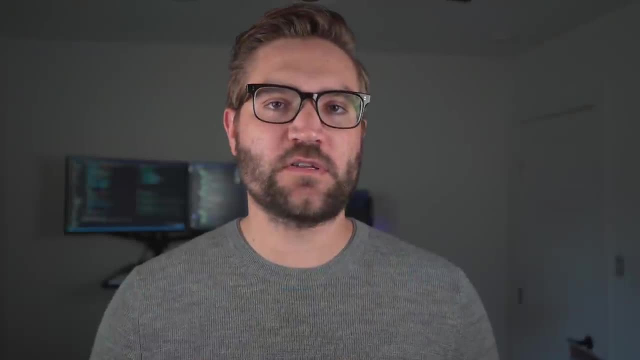 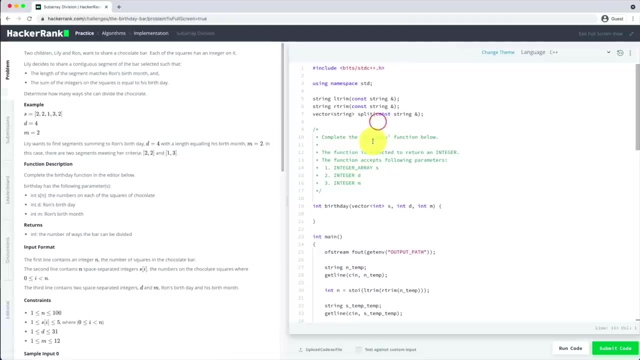 You really want to make sure you know exactly what you're focused on for that session? I mean, if you're newer to this, I can give you a really easy suggestion. I noticed a lot of you guys who start doing hacker, rank and leak code problems just struggle with understanding what the problem. 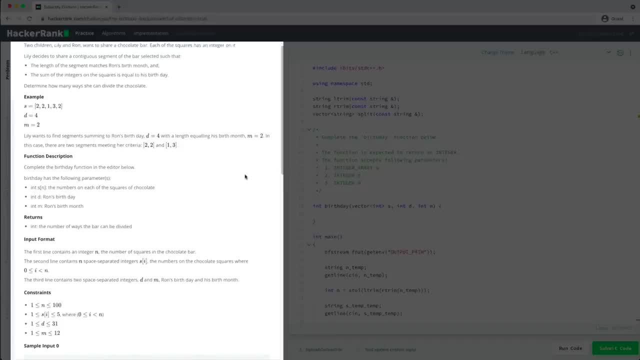 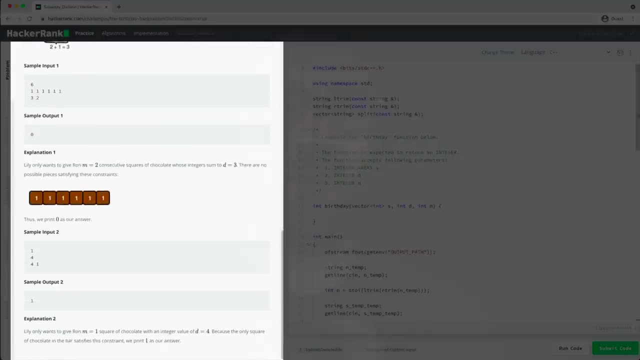 is asking. So what you can do when you sit down to study is really say: okay, I'm going to sit down and really try my best to comprehend what the question is asking. So I'm not even going to write any code, I'm just going to maybe go through one, two or three problems to try to understand. 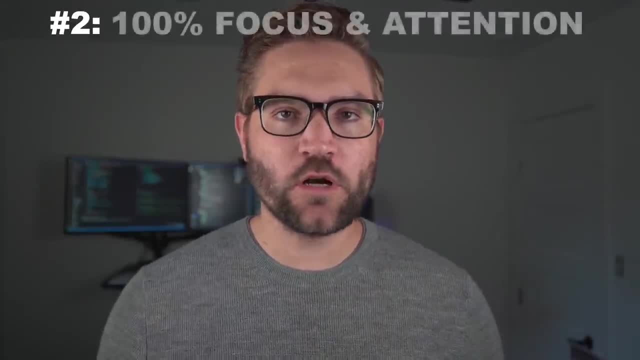 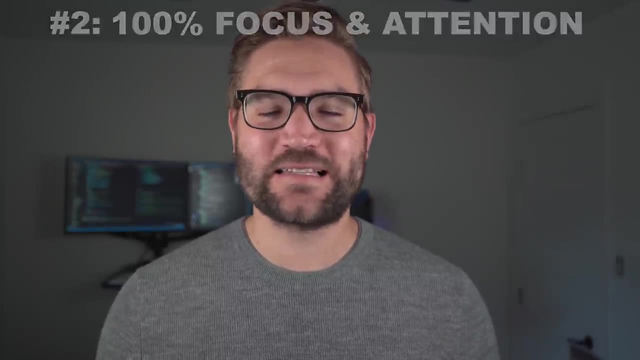 what they're asking. The second part of deliberate practice is that it requires your 100% focus and attention. So if this is something that you can do while you're watching a YouTube video in the background, listening to podcasts, that's not the type of practice that you want to get into To get 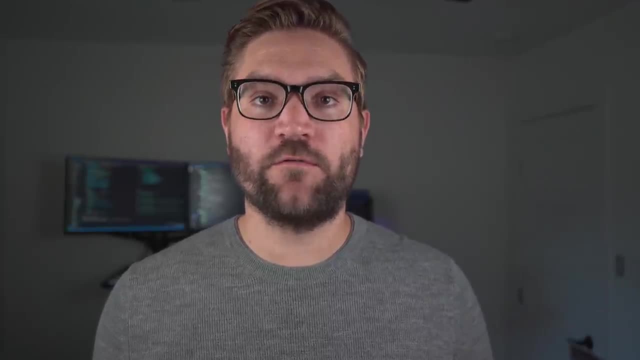 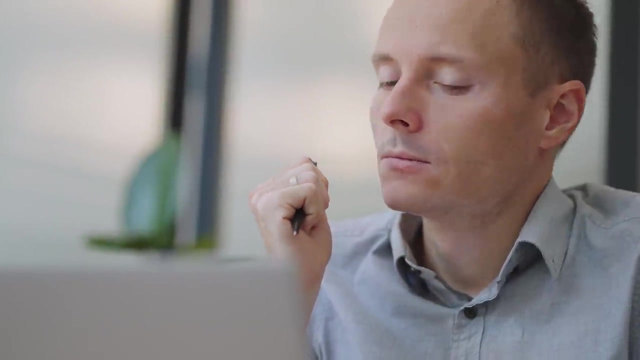 the most out of something like building a portfolio project. you often have to go very deep into thought. Maybe you are thinking about what code you should write next. Maybe there's a bug that you ran into and you have to really think deeply and really analyze your code. But that's going to. 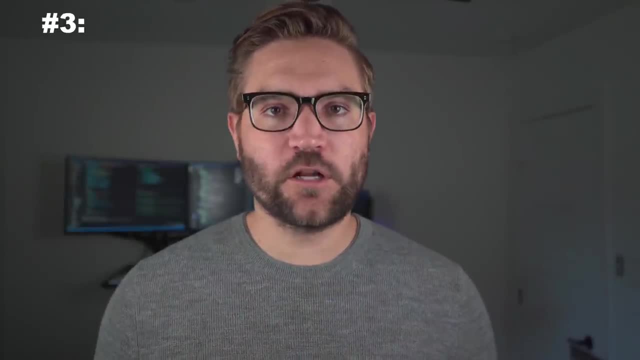 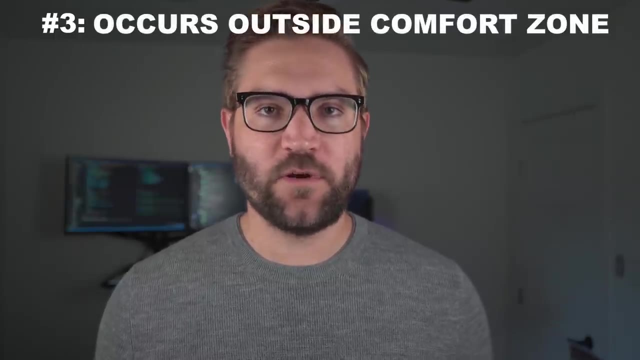 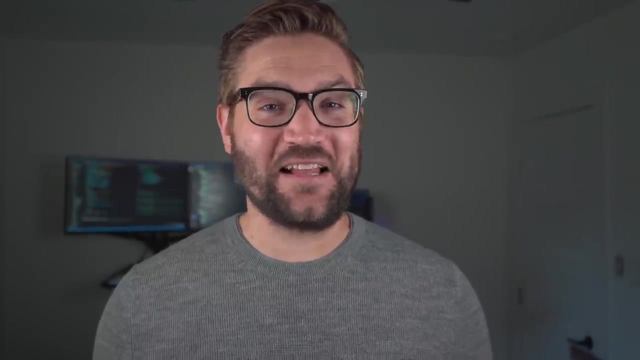 require you to have long periods of thought and concentration. The third component of deliberate practice is that it requires going outside of your comfort zone, And this is so important. Everybody loves to show up and practice on the things that they're good at. Nobody likes to show up and practice on the things that they're not good at, because you're going to. 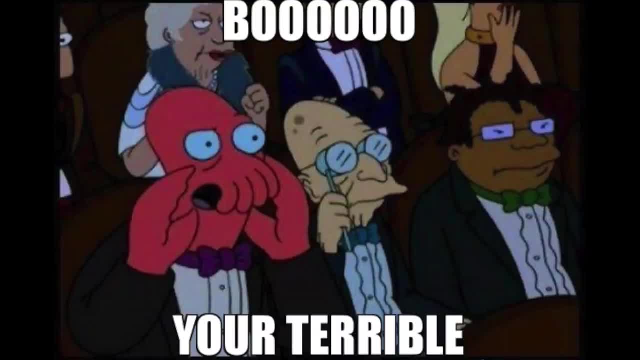 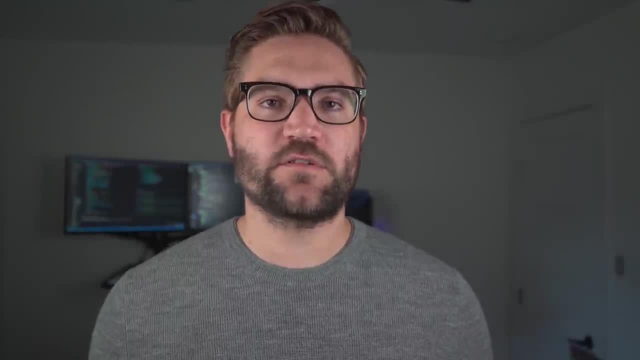 get a lot of feedback that, well, you're not good. I mean maybe even that you suck. But if you're ever going to go beyond a basic understanding of programming, you have to feel uncomfortable. Let's say you're learning JavaScript, for example, A common, difficult concept that you're going to 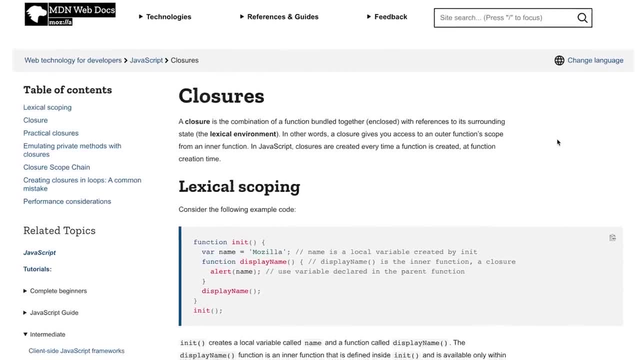 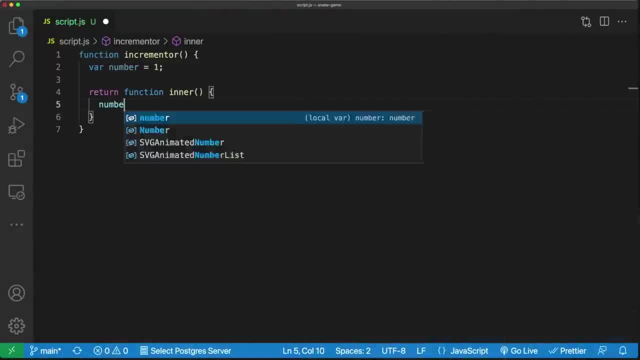 run into at some point is closures. Now you're going to read some articles about closures, watch some YouTube videos. That's going to be very comfortable, But what's very uncomfortable is taking that knowledge you've learned and then applying it in some way, So maybe using it in an 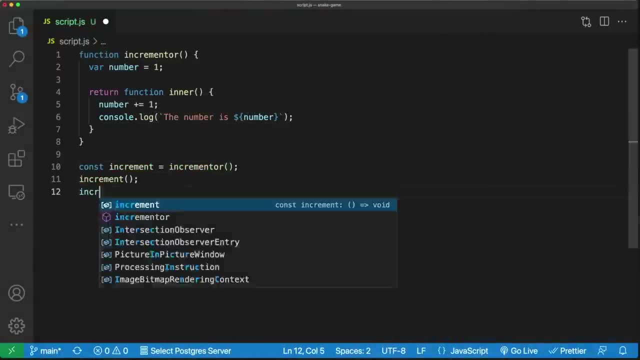 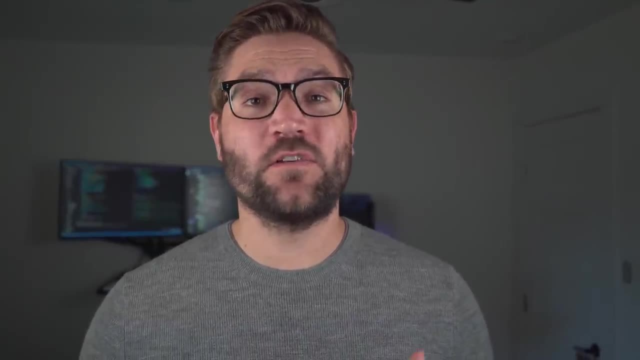 actual problem somewhere. But if you don't do this and push yourself outside of your comfort zone, then you're always going to just stay exactly where you're at. So those are the key parts of deliberate practice. If you want to learn more about deliberate practice, I'd actually recommend 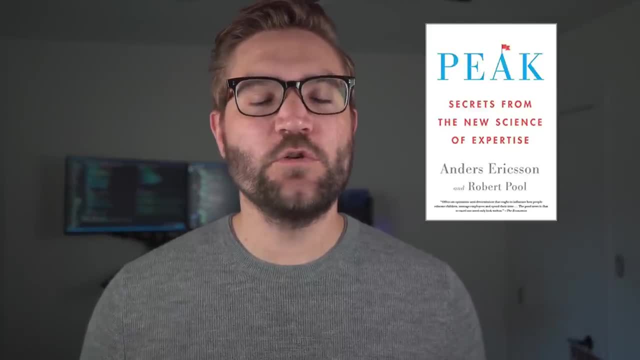 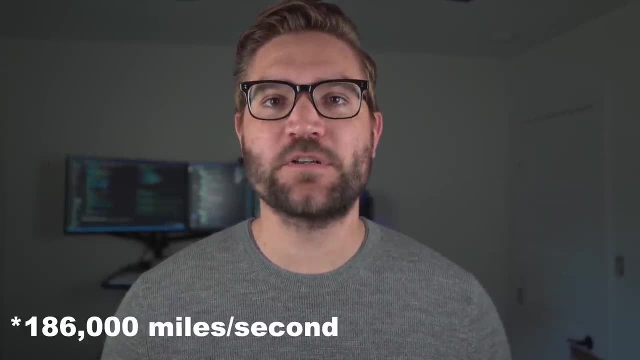 checking out Anders Ericsson's book called Peak Secrets of the New Science of Expertise. Now, while we're on the subject of speed, I want you to move at the speed of light, which is 186,000 miles per second, down the page to smash the subscribe button. 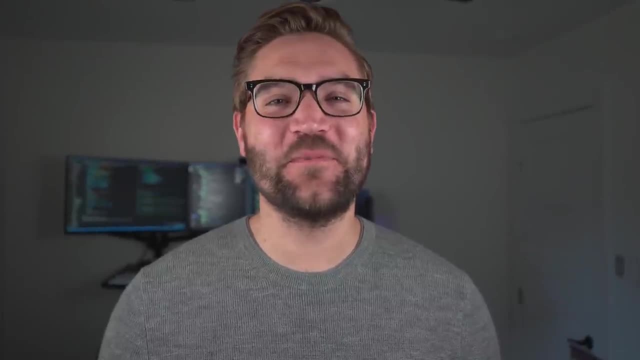 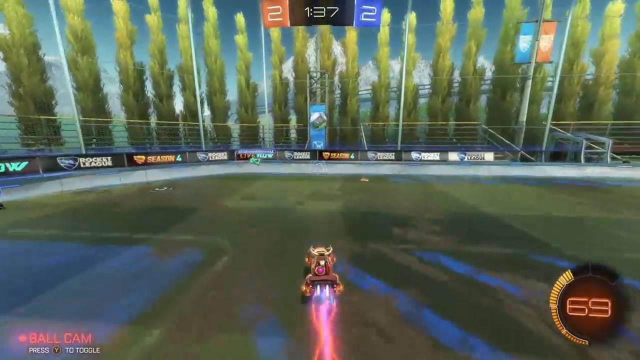 It's greatly appreciated. Okay, so the next principle to implement in your approach to learning to code is actually something that I learned from playing video games. During the pandemic last year, I fell in love with a video game called Rocket League, And the concept is: 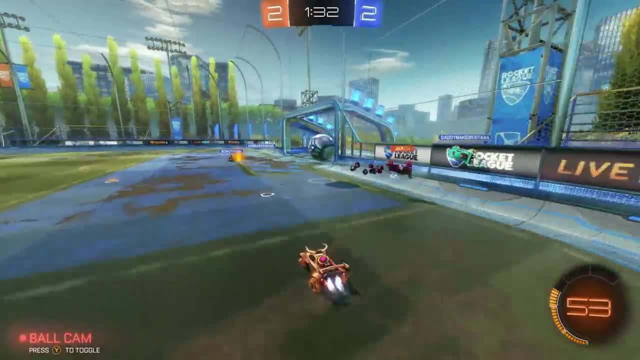 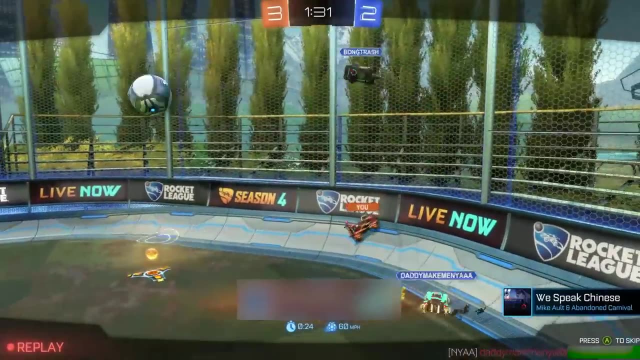 really simple. It's basically you get to play three on three soccer matches online with other people, But instead of controlling little guys on a field, you're actually controlling little cars that try to hit a ball into a goal. The game was actually a lot of fun for the first. like one to 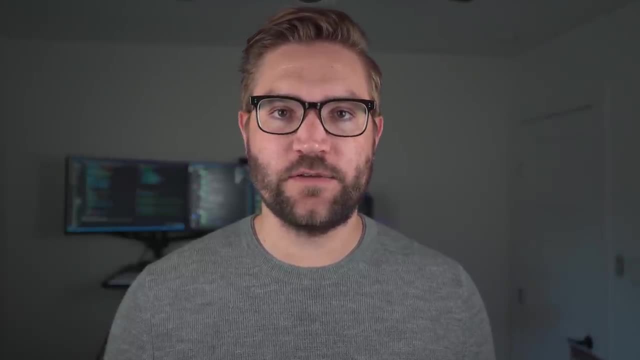 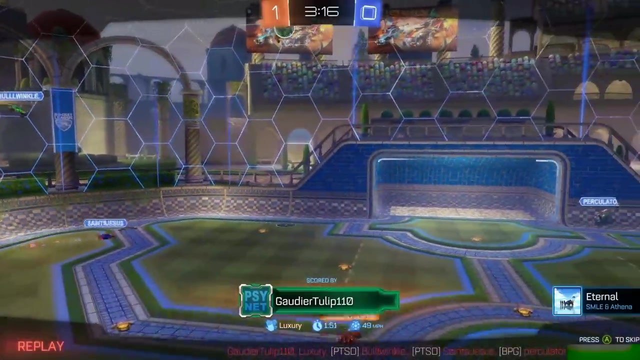 two months. But then I started getting frustrated with my lack of progression in my skills. And you see, there's a skill specifically I started to notice in the game that really can make you better. See, in the game you can actually jump up in the air and, like shoot your car through the air. 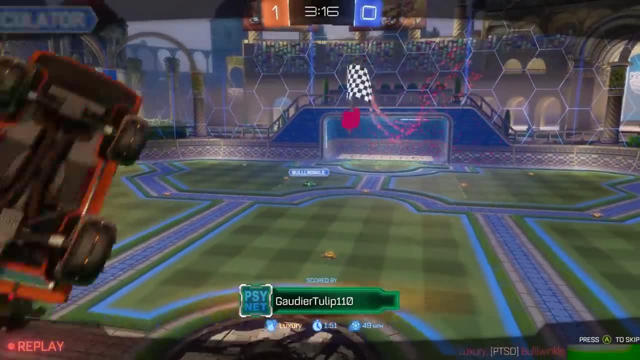 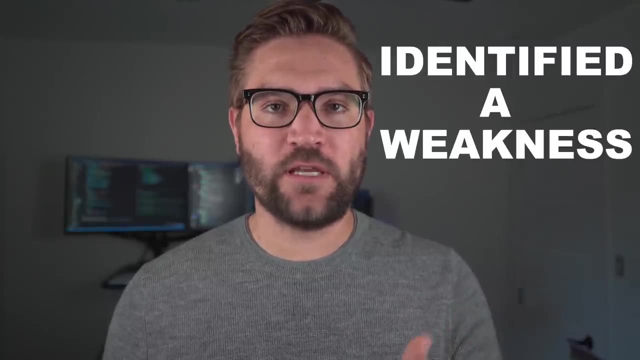 so you can hit a ball into the goal. It's called an aerial. It's very, very hard And I noticed that a lot of the better players I was playing with could do that. The key thing that I did here was I identified a weakness. So, moving forward, I knew if I wanted to get better, I had to get. 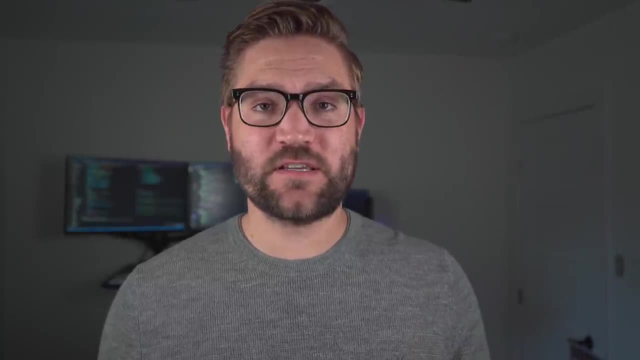 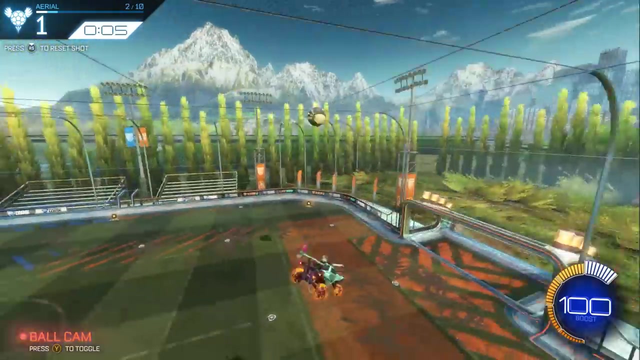 better at aerials. So instead of playing these three on three matches all the time, instead I would just sit there and I would practice and I would do some of the drills that you could do, where you could just jump up and hit a ball that's in the air over and over again. 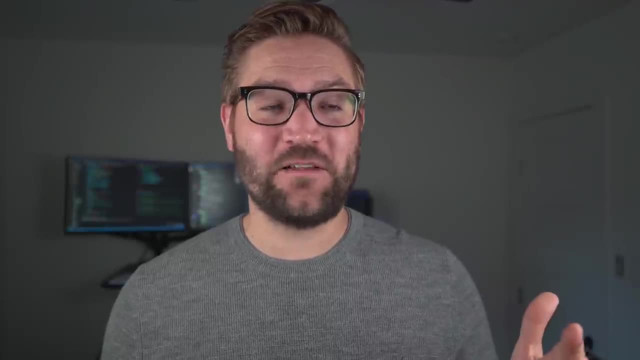 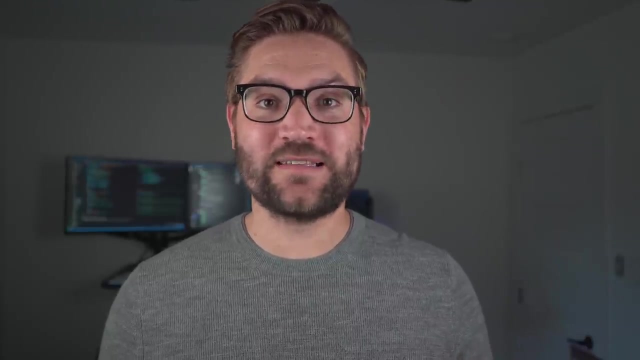 And you want to know something. It was actually really terrible, Like at first. I could barely hit like maybe one out of every 10 balls in the air, but I did it for a couple of days. I then moved it onto a couple of weeks And the interesting thing happened: I got better. I was 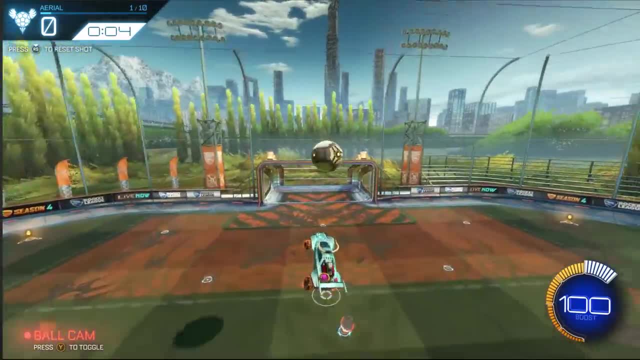 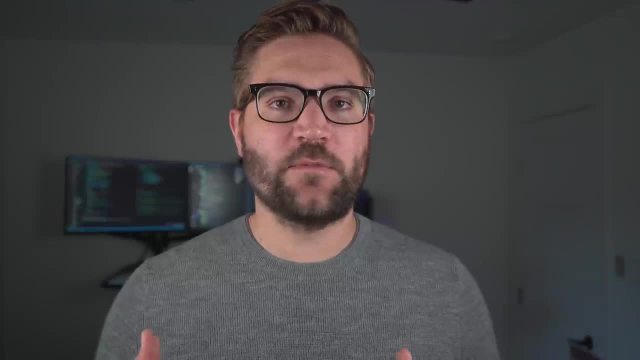 hitting, you know three or four out of 10 balls in the air, And when I would play those three on three matches, I suddenly was playing a lot better. The important principle I'm demonstrating here is attacking your weaknesses directly. This concept actually comes from one of my favorite books on 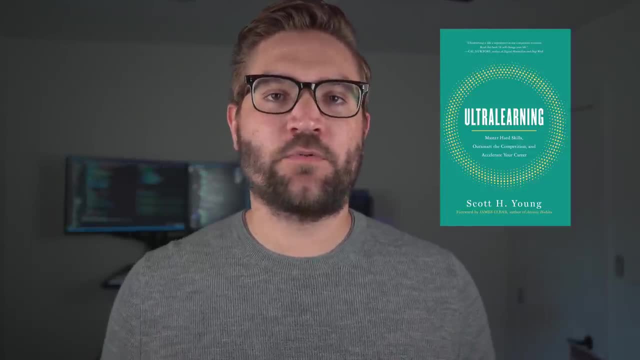 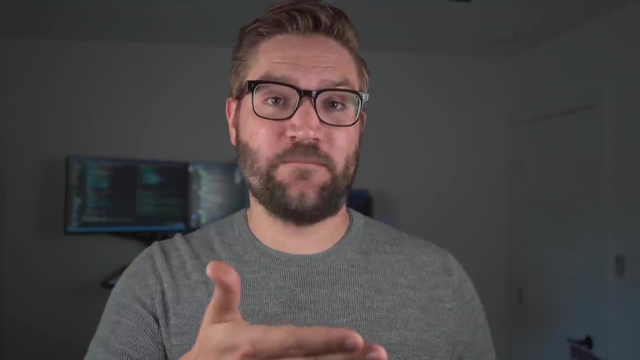 programming, and that is the book Ultra Learning by Scott Young. Taking this back to programming, you will likely encounter concepts or problems that show you where you are either weak or where you lack understanding, One of the most common places that new JavaScript developers are weak. 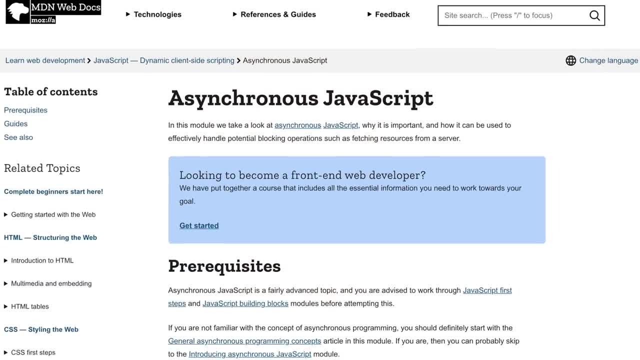 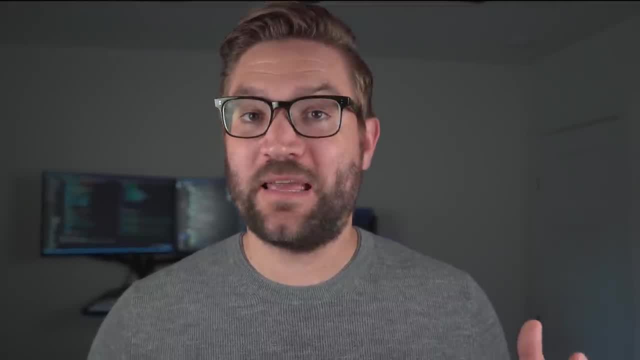 at is really their understanding of non-blocking, AKA asynchronous programming. So if you've worked with promises in JavaScript, this is what I'm talking about Now. when most people run into something like promises, they can make basic sense of it. They can use it in a problem to. 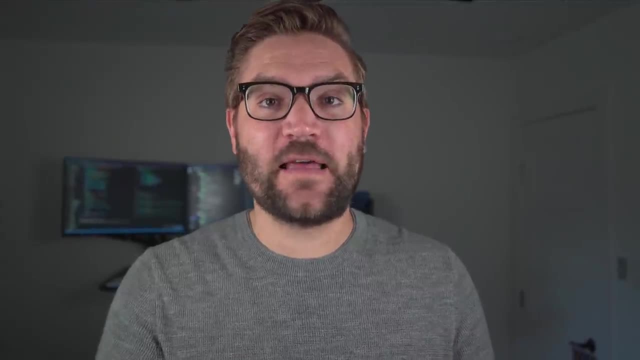 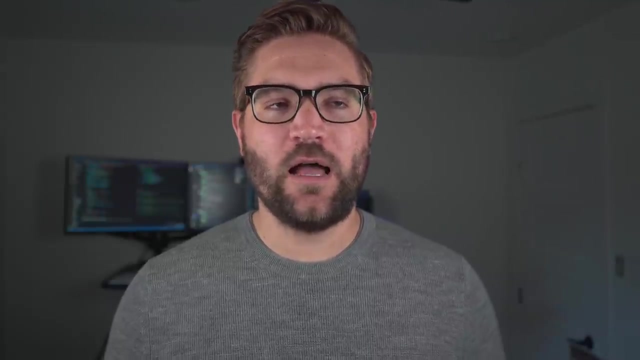 get a desired outcome, But if you ask them to do anything more complex than that, that's where they really run into a wall. If this happens to you, it's a huge opportunity to attack this problem head on. Now, how do you attack something head? 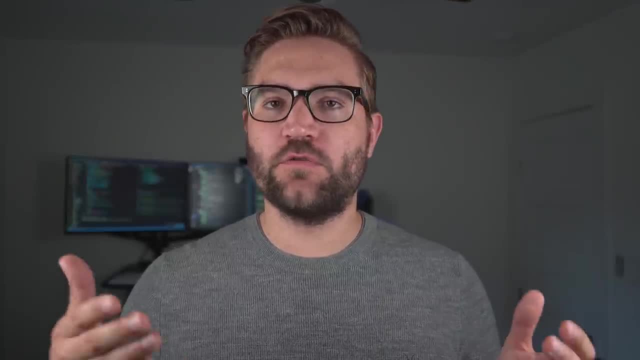 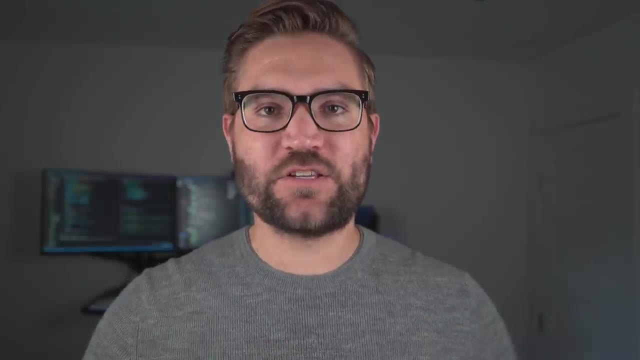 on. Once you've clearly identified a weakness, like understanding promises, then you can do one of two things. The first thing you can do is you can make note of it. There are going to be times when you're working on something, you recognize a weakness and you can't just stop what you're. 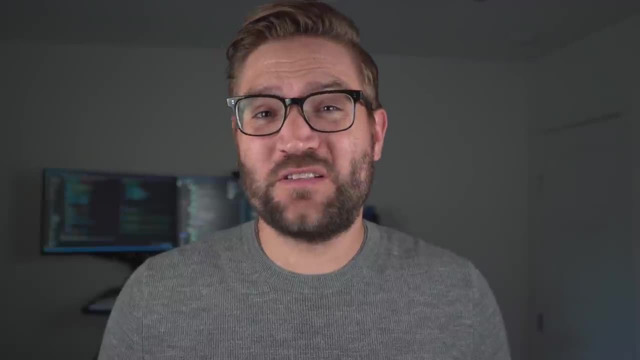 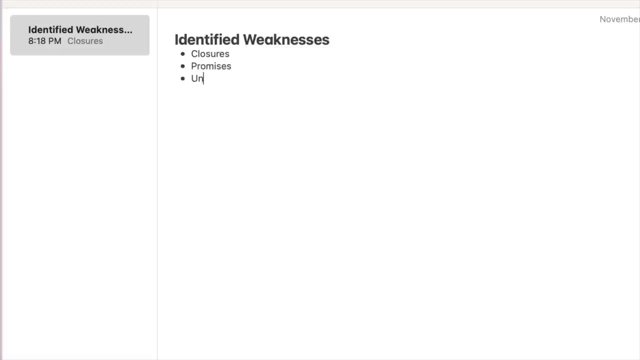 doing to really drill and focus on that weakness. So the best you can do is basically make note of it. So I actually recommend creating a Apple note, a Google document that really lists out all of the weaknesses that you run into and you want to regularly update and drill them when you 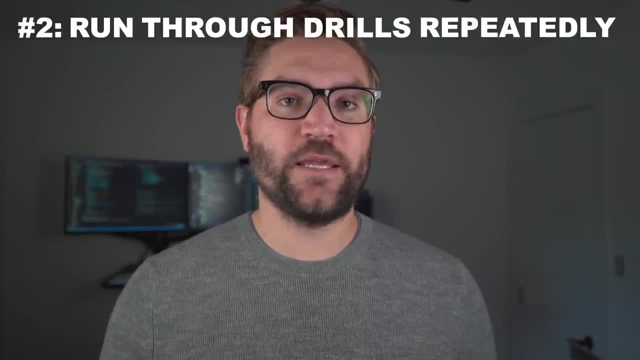 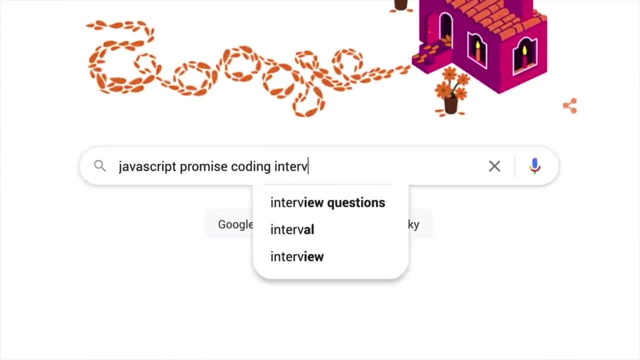 have time. The second thing that you can do is to run through drills repeatedly. So for something like the promise problem- not understanding promises- you can Google something like JavaScript promise coding interview and see what some of the questions that pop up. You can run through all of. 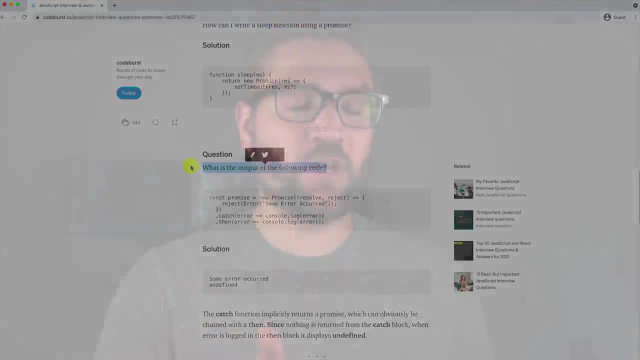 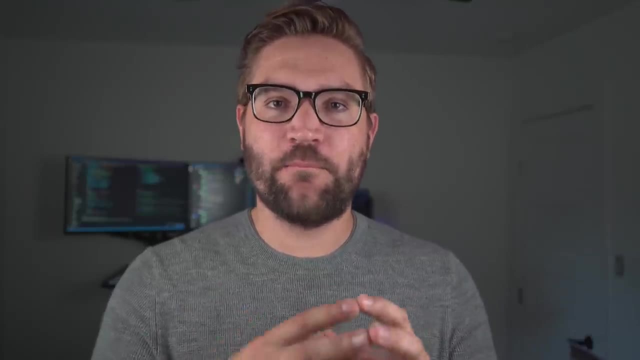 those And really the key of what that's going to do is it's going to allow you to work on different problems in different contexts repeatedly, over and over again, And eventually your understanding of it gets better and better And, honestly, this principle has probably been the one thing that has sped up my results. the 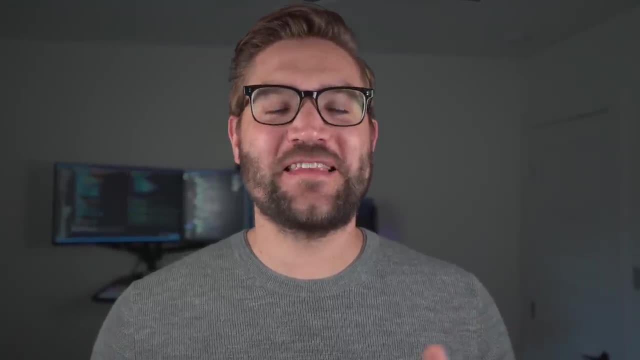 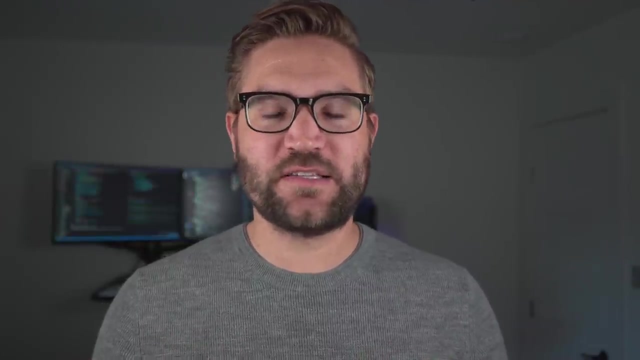 quickest. Okay, So if you followed everything I've laid out for you so far, then this next part should be the icing on the cake that brings everything together Now, despite what you see in popular culture, where success is just about grinding and hustling and working more and doing, 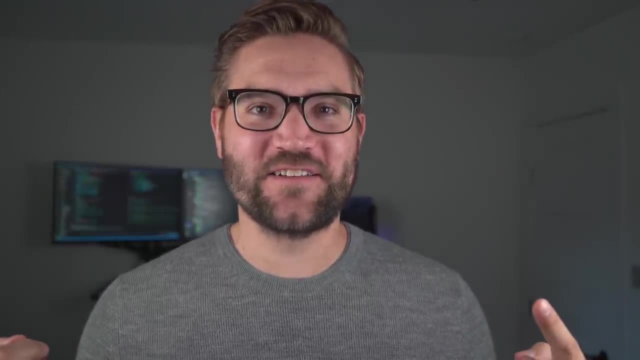 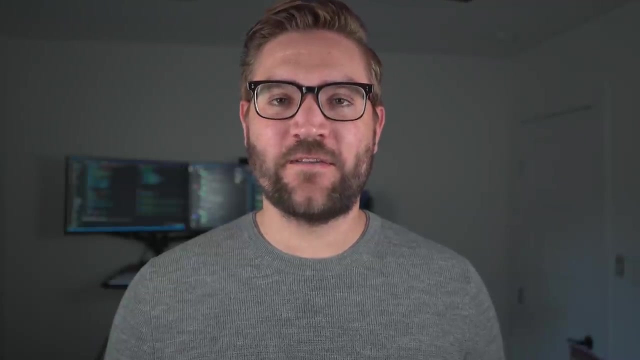 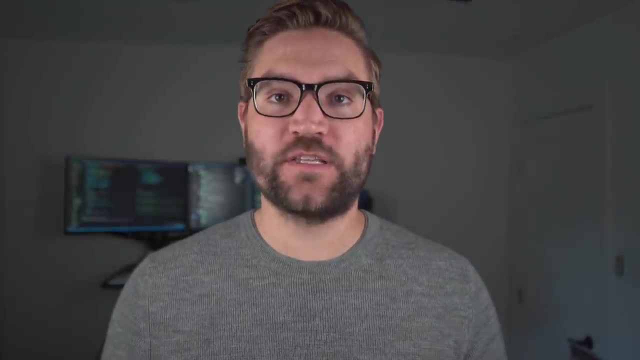 more and intensity right Like cue the Rocky training montage. No, that's definitely not the key to success. I'd say that the key to rapid skill development is that you must treat your brain and your mind like an athlete treats their body, So just like an athlete would never put in a hundred hours of 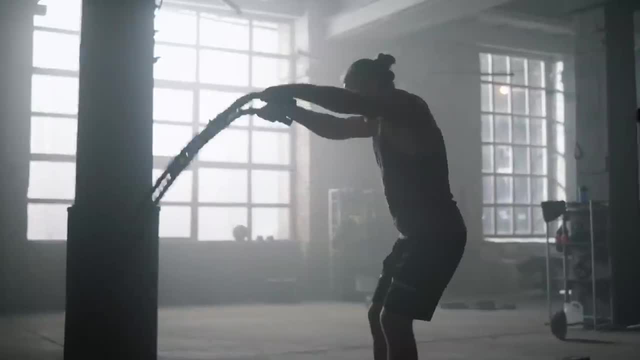 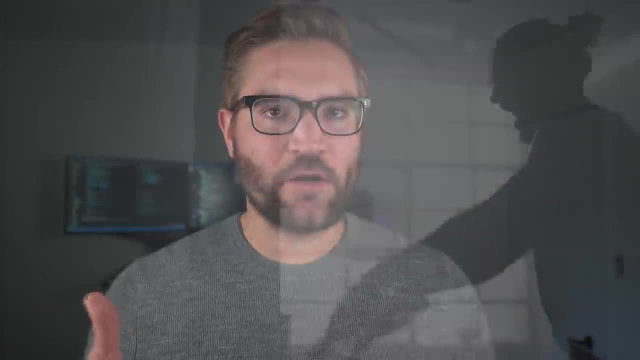 intense training per week. neither should you. In fact, most athletes know that the secret to success is really short but high intensity training sessions with a very long periods of rest. Now just imagine how tired an Olympic athlete would be after one or two hours of intense. 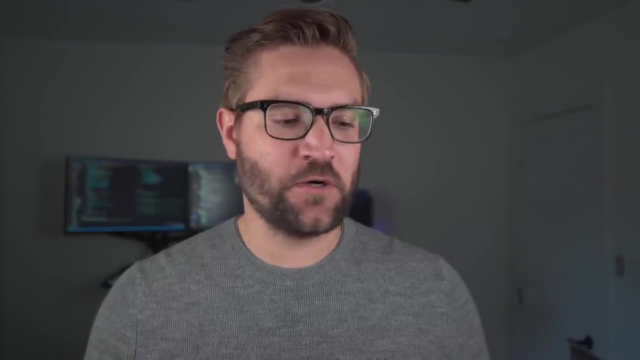 training. Well, if you're listening to the advice so far, where you're going to be outside your comfort zone, where you're going to be A hundred percent focus, where you're going to be doing drills repeatedly, over and over again, Well, 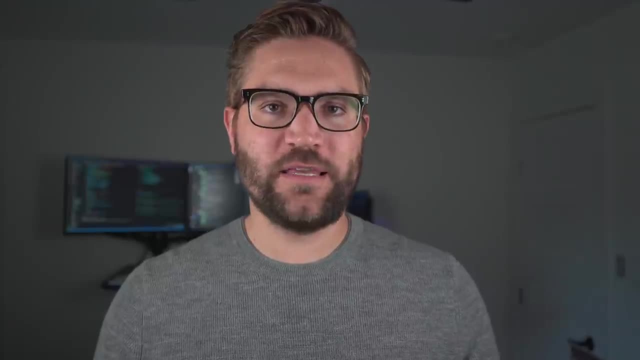 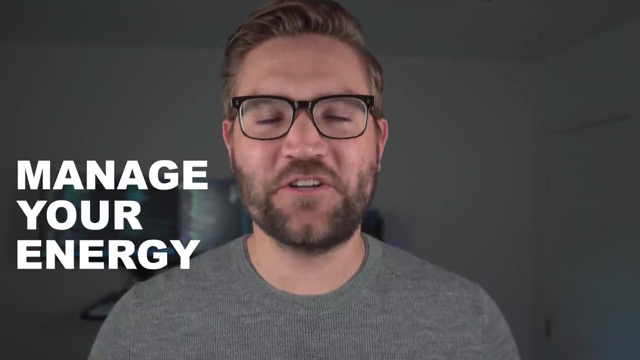 you should be really tired at the end of every day. So my last point here would be that, if you are going to maximize every ounce of effort that you put into this, it is critical to learn to manage your energy levels effectively. As far as energy management, there are a few simple. 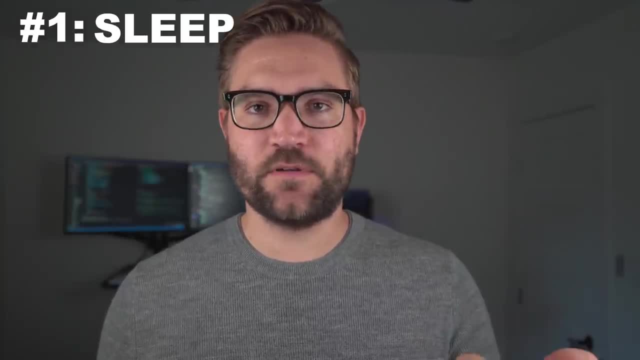 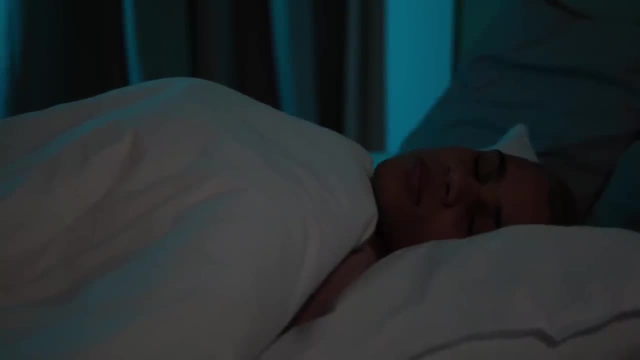 guidelines that I've seen work really well for people. The first one is sleep. So you have to make sure that you're getting your seven or eight hours of sleep per night to really recharge the batteries. The problem that you really see when start coming back on sleep is that the part of the brain that regulates emotion, that really 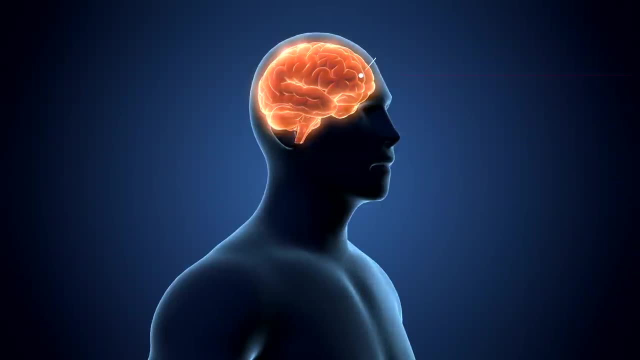 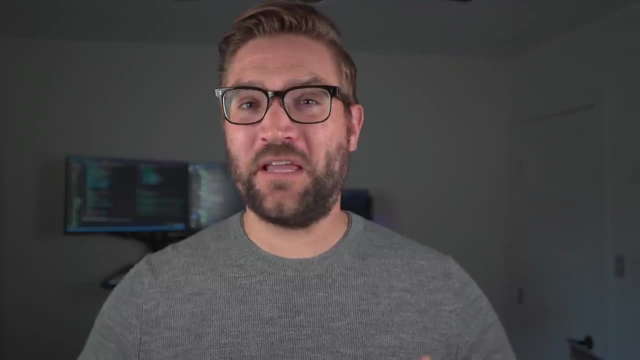 helps you to maintain your discipline and show up weakens. right, That's called the prefrontal cortex, And the problem is is that if you're not recharging your batteries the next day, you're going to be grumpier. You may not actually sit down to do the work, And if you actually do the 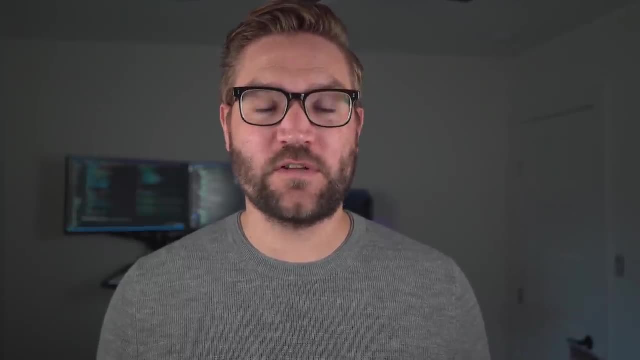 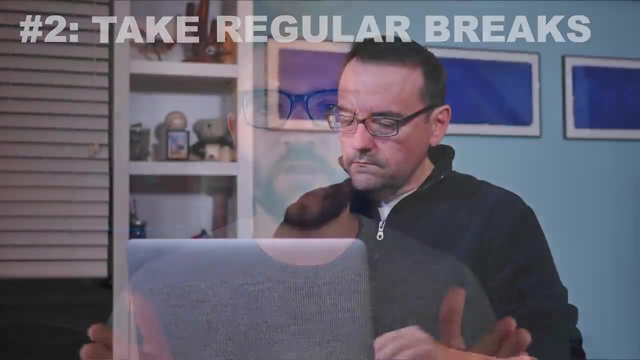 work, you're less likely to be able to focus for long periods of time. From there, the next thing to keep your mind functioning at its peak is to take regular breaks, right. So if you run into an impasse, you're working really hard. it's very tempting to just keep pressing and pushing. 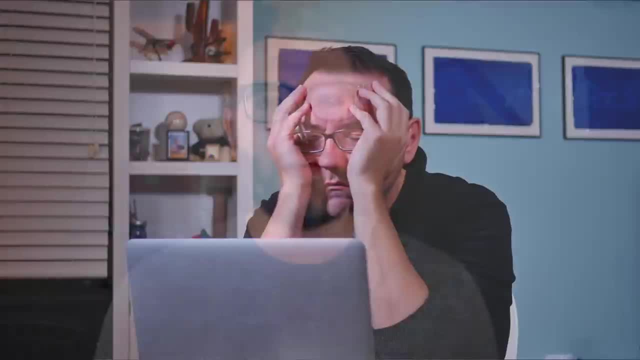 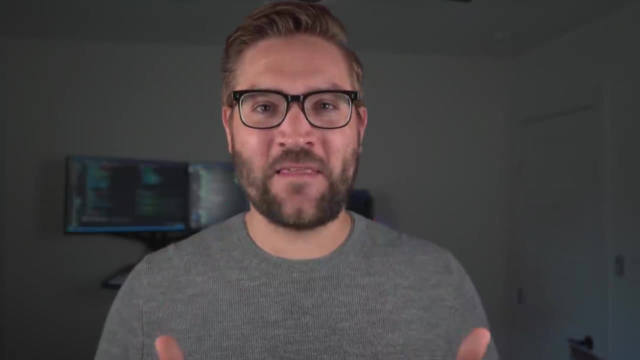 on and working for another half hour, another hour, But in all reality those are really good times to take a break. There's something called diffuse thinking, So there's actively thinking about something and then there's actively thinking about something and then taking a break, and 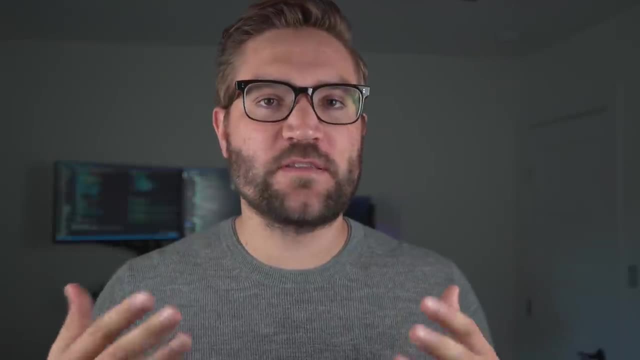 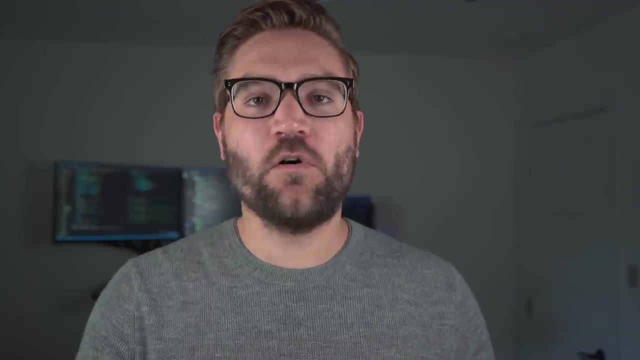 letting your brain just kind of think about things in the background, And one of the coolest things about this mode of thinking is that you can actually problem solve and be very creative when you're not thinking about things. So you want to take breaks for that reason, but also because you 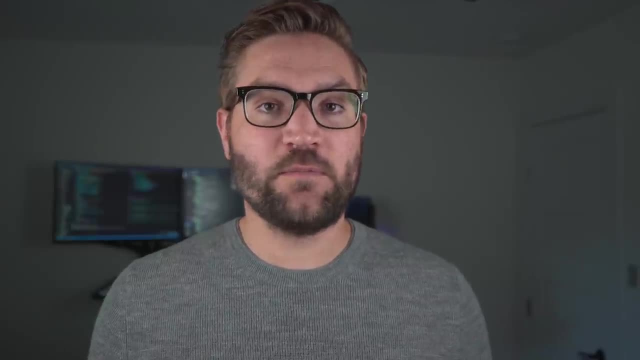 just need to recharge your batteries. Often, I'd even say as far as study blocks, make sure you're not studying for too long. So if you're going to study, let's say six hours in a day, don't study six hours straight. Maybe break that. 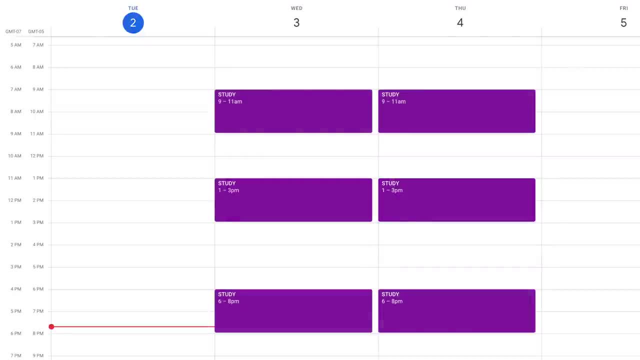 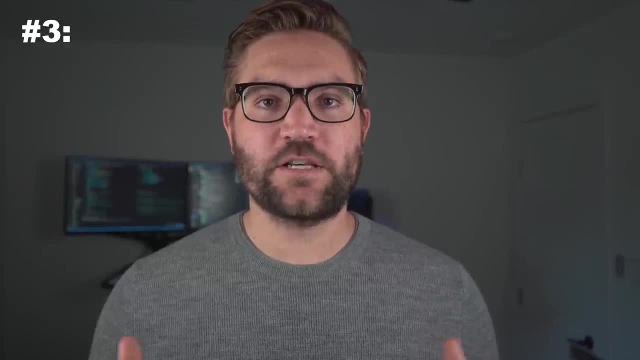 up into three blocks of two hour study periods. That's really how I approach things. I never try to cram things in and it really keeps my mind fresh and I have much more energy because of it. The last thing that I actually personally recommend for energy management is just regular. 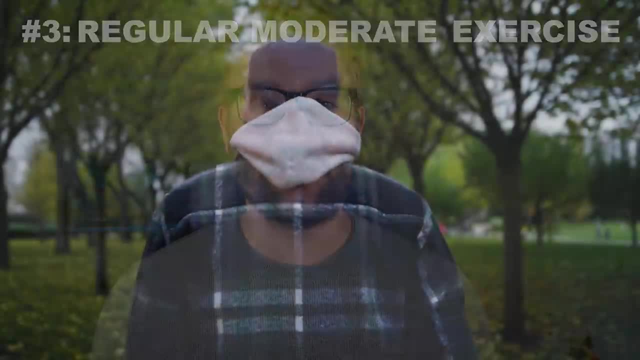 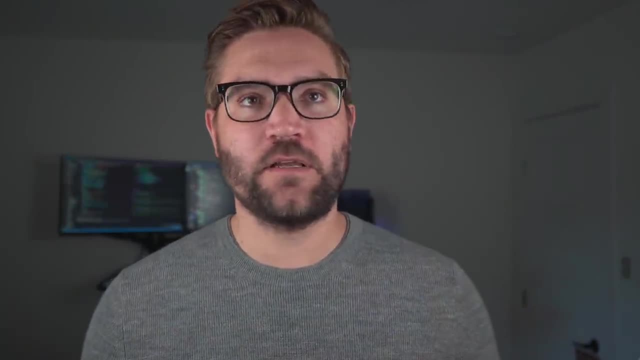 moderate exercise. So that could even just mean something as simple as walking around the block a few times per day. I personally recommend about 10,000 steps for this, but it could also be a weightlifting regimen, It could be a running regimen, It could be doing. 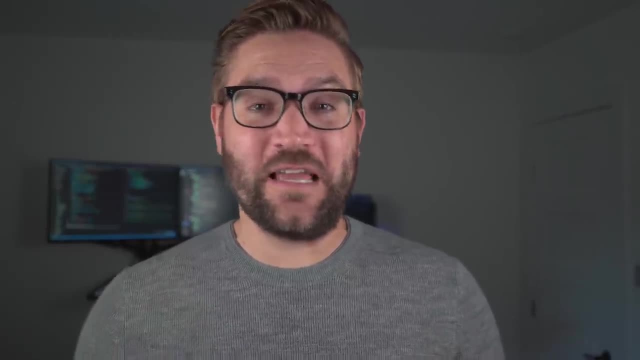 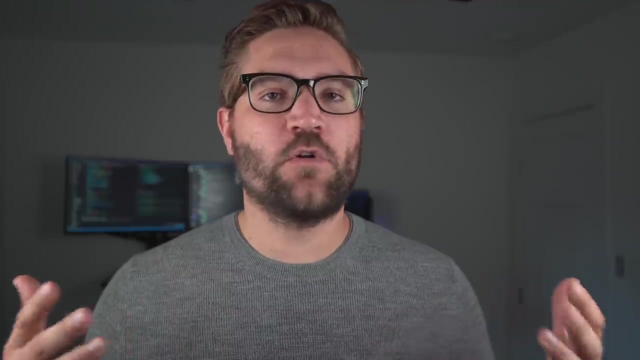 something like yoga. The key component of this is make sure to get your body moving. If you can get yourself outside, that's a plus, but the more that you can get sort of blood flowing through the body, it will honestly do wonders for not only your ability to think but also for your 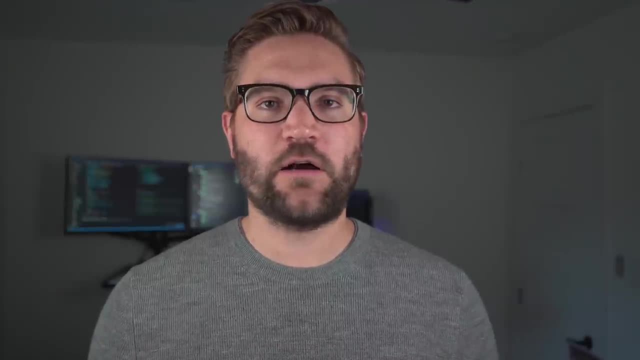 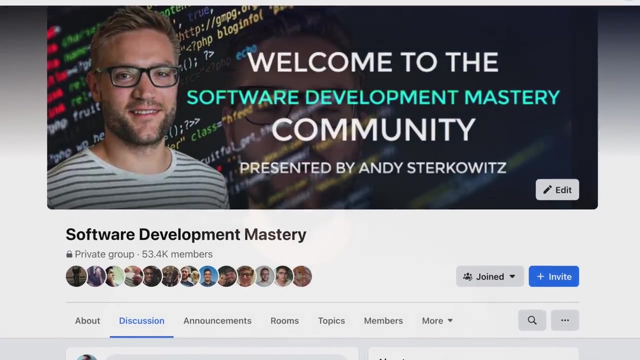 ability to come up with creative solutions. Now, in addition to everything that I've laid out for you here, if you're looking to join a group of like-minded people, then come join my free Facebook group. I will leave a link in the description below of how you can do that. 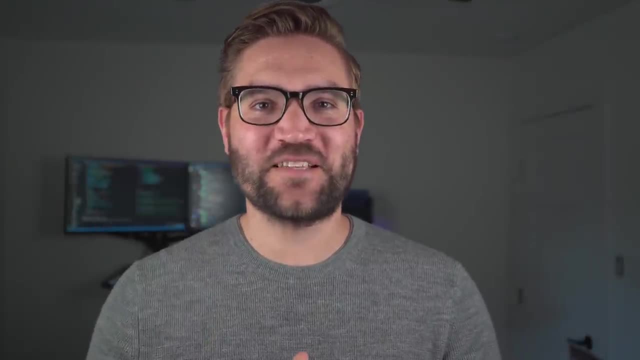 Other than that, thank you so much for watching And, as always, peace out. 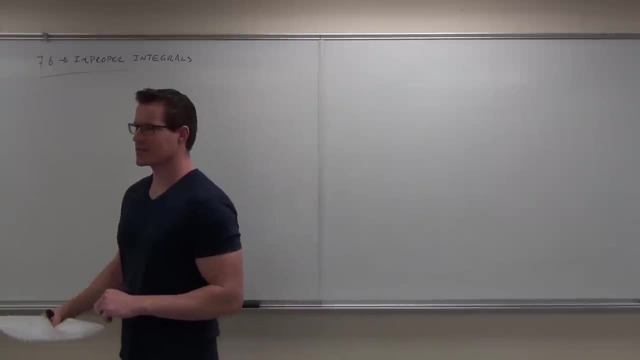 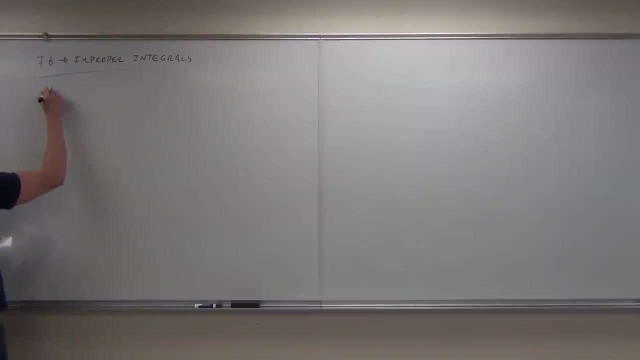 So improper integrals. my goodness, what in the world does this even mean? Well, typically, what we need for integrals to work So normally, for any sort of definite integral, from like a to b of some function, what has to happen for this to exist, for us, before, right now, For this to exist, and let's 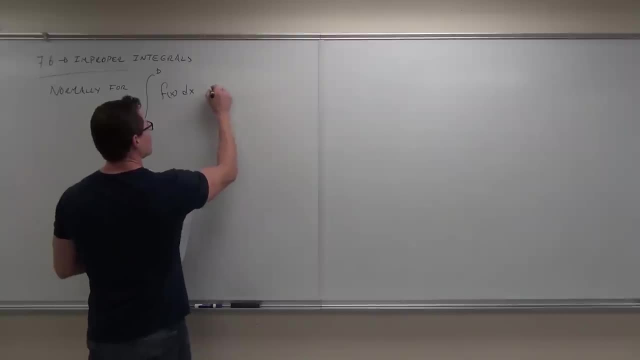